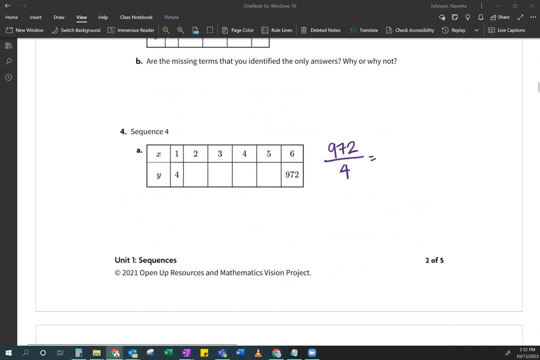 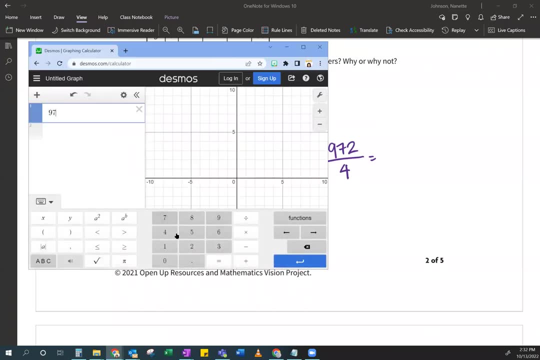 Yes, Ms Johnson. Okay, so I do that. Let me pull my calculator because I, off the top of my head, I don't know what 972 divided by four is. So here I say 972 divided by four and it says: oh. 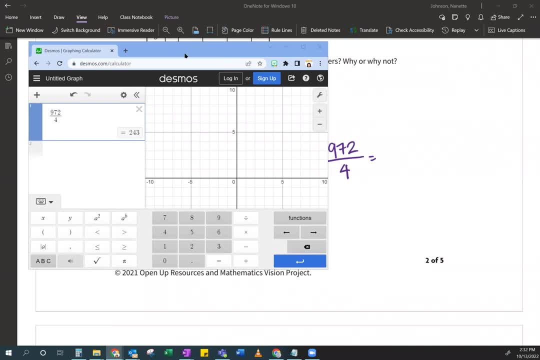 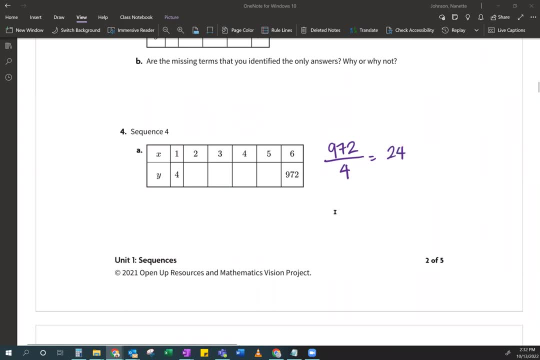 it's 243.. Okay, move that real quick, So that's 243.. And then we talked about: okay, well, because I have this many jumps, and in this case it's 123.. Two, three, four, five. I know you guys are like Ms Johnson, you're counting with me, Yes. 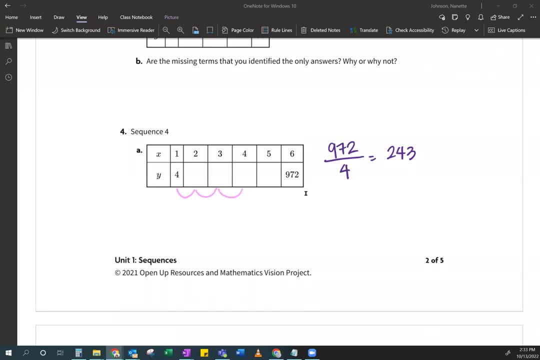 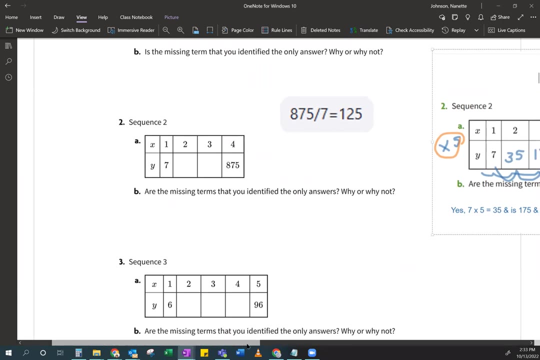 because it's very important that you know how many jumps we have. So we have five jumps, And so what the jumps are going to tell me is who is sharing this 243.. So then, what we talked about was we needed to write this equation, right, This equation that kind of looked like this something: 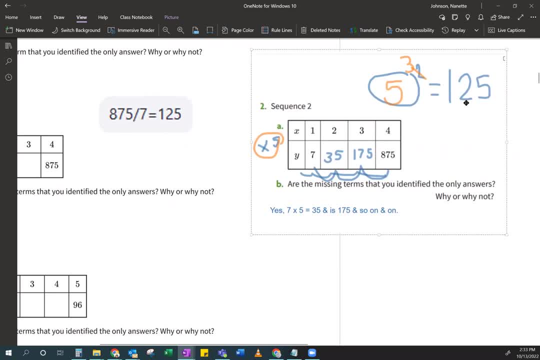 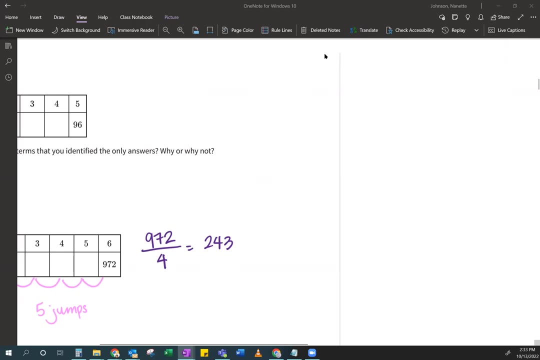 to the third equals to 125.. So 125 came from the fact that we divided. I got that. The three came from how many jumps we have. Oh, so in this case it's five jumps Exactly. So we want to move this and make it a little. 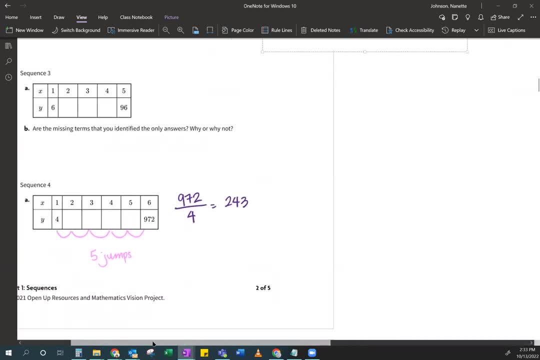 smaller so I don't have to move my screen. Okay, So I want to figure out. so you want me to write an equation with that five as the exponent, Exactly. So I'm going to put a five as the exponent there, And then I'm going to put equals to 243.. And I'm looking for this number. that goes. 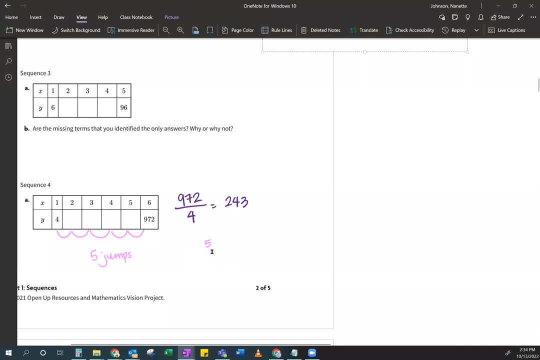 right in here. So I'm going to write an equation that has five as my exponent, And then I'm going to write equals to 243, because that's what it's equal to. Let me think of this really quick, Right? So then I want to. 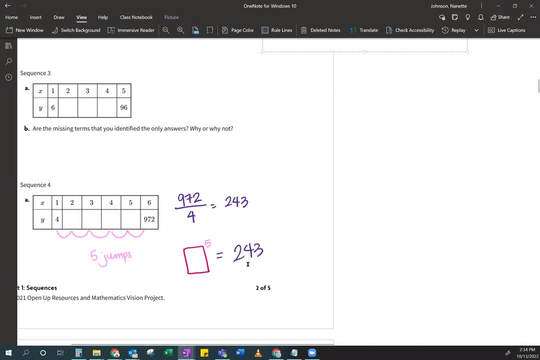 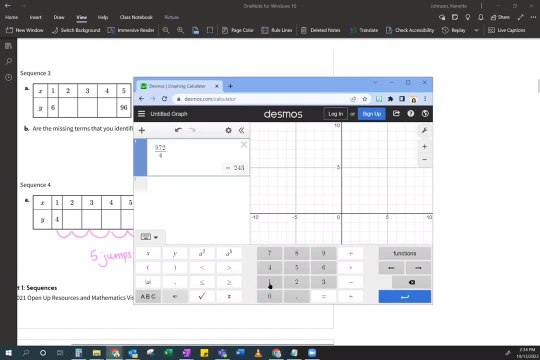 look for what number to the fifth gives me 243.. So in case you don't know what that actually means on this calculator, right? In case you don't know how to do that on this calculator, no problem, I'm just going to start using numbers. I'm going to start with the number I don't know: five. 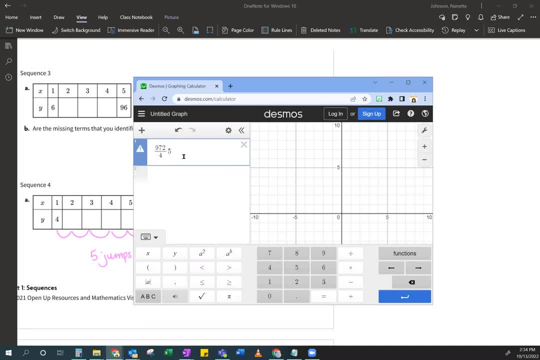 So five to the no no. Now, the reason why I'm using five is just because it's the number that came into it. I actually know what to the fifth gives me 243, but I'm doing this for you all, Okay. 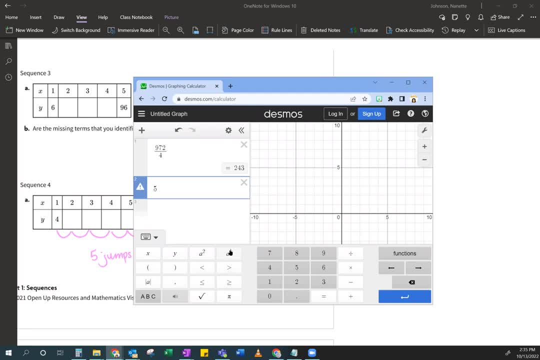 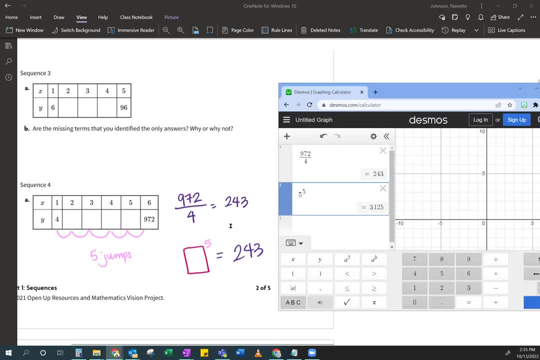 Five to the fifth. Here's two that right here. See two. the fifth: Oh, that's 3,125.. That's way too big. You see how big that is. That's. that's too big, So I need to go smaller. So let me try two. 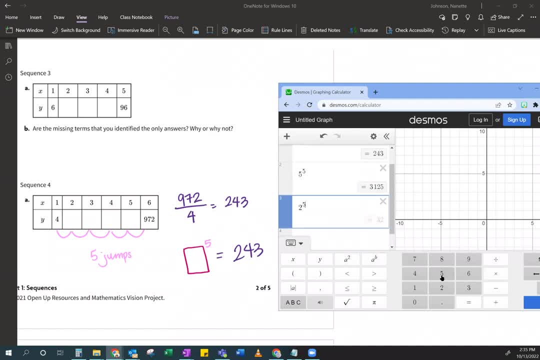 So two to the fifth, Oh, that's 32.. It's too small, So let me go like. this is kind of like the Goldilocks thing: This is way too big, This is way too small, Oh, this is just right. So I'm. 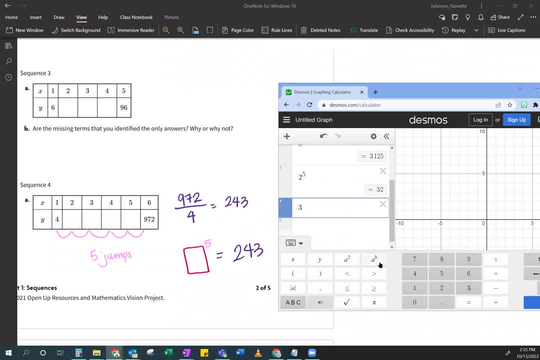 looking for the number, that gives me 243.. And then I'm going to write equals to 243.. And then I'm going to just write: So let me try three. three to the fifth. Oh, it's 243.. Okay, So what do you want me? 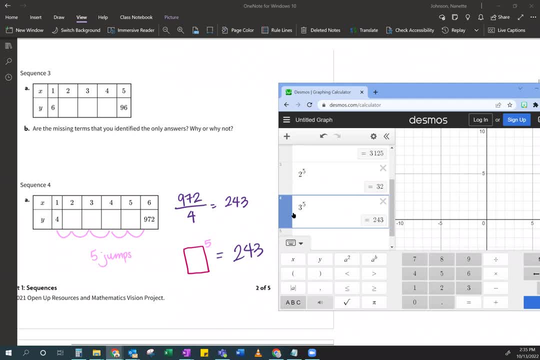 to do, Ms Johnson, So that three is now called our common ratio. It is our common ratio, So let me write that down: Common ratio. So what, Ms Johnson? who cares if that's our common? oops, sorry, Who cares if that's our common ratio? Well, our common ratio. 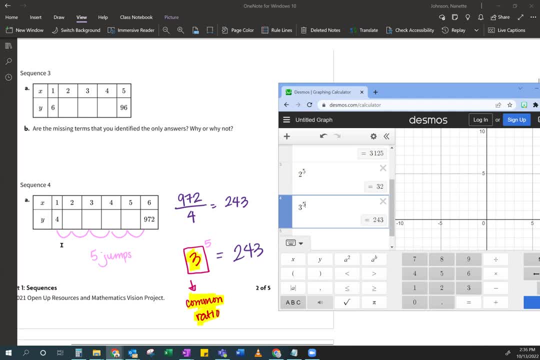 right is the number that belongs right here, And we multiply by three to get to the next term. by three to get to the next term. by three, to get to the next term by three, by three, by three, Very good, Okay. So, Ms Johnson, you want me to multiply by three? Uh-huh, So what I'm going to? 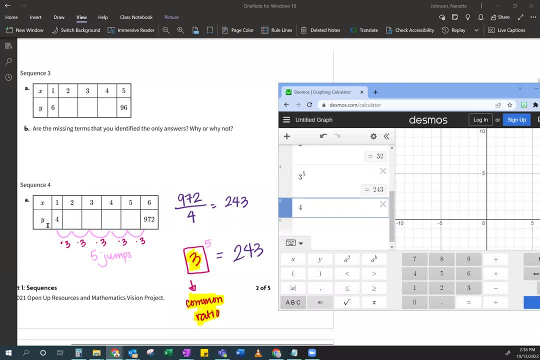 do here is: I'm going to start off with our first guy, which is four, and I'm going to multiply him by three. Oh, it gave me 12.. So you want me to put 12 right here? Yeah, So I'm going to put 12 right. 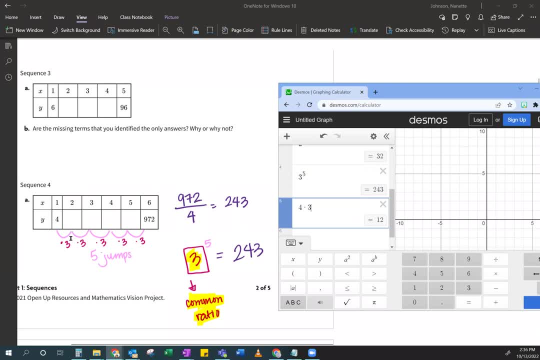 here, Ms Johnson, Yes, So you want. I'm going to put 12 here, Exactly. So then how would I get the next term? Well, you would just again multiply by three. So as this thing catches up, 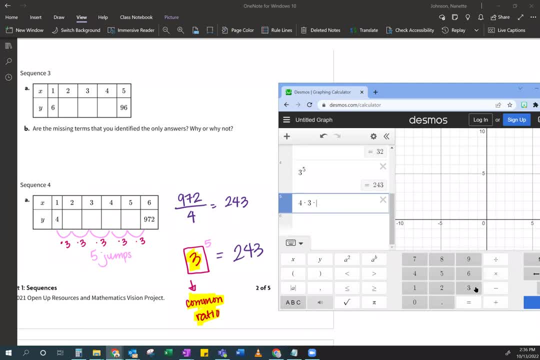 to me. I'm just going to multiply again by three. So multiply by three and then I get 36.. So I'm going to write that in there: 36.. I'm going to hope that this guy catches up to me eventually. 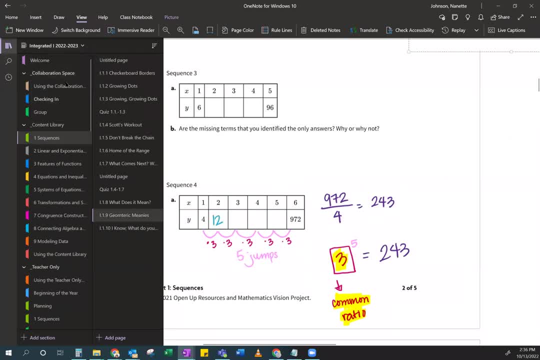 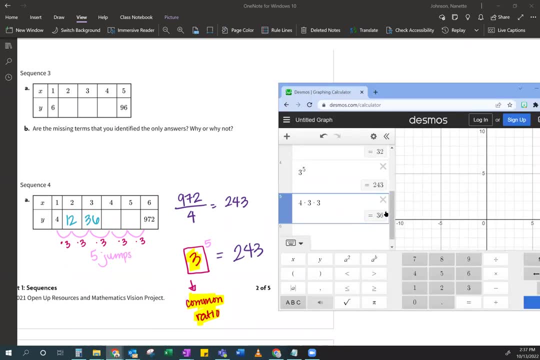 If he doesn't, no problem. Yep, There you go. Okay, So then let me grab my Desmos again. I'm going to just keep going. So then I go times three again, So that's 108.. And then time: oops, not three. Oops, my bad Back up. Sorry, Sorry, Sorry. 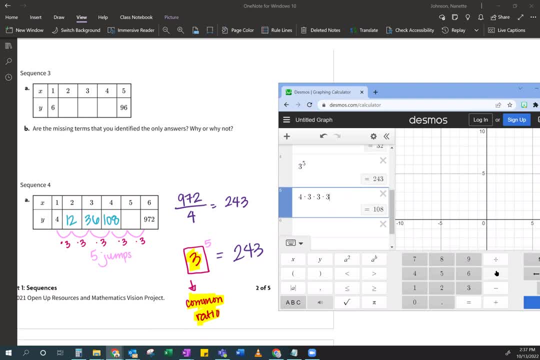 Sorry. So then I want to go times three again, and I get 324.. And then I go again, And then I get 972.. And I'm so excited right now because, look, that number matches that number. And then my four matches my beginning, And I have one, two, three, four. 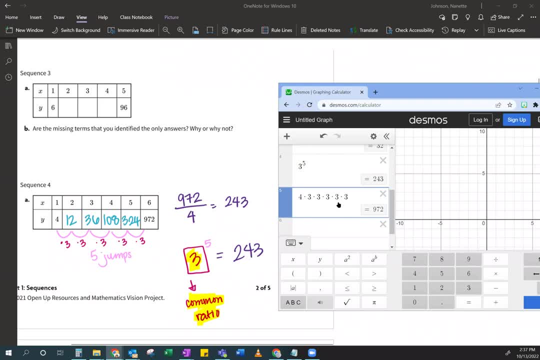 five jumps, And I have got one, two, three, four, five jumps. Now there's other ways that you could have filled all this out, but this is kind of like the recursive way And because I already had my starting point and I had my common ratio, I just thought: why not? Okay? 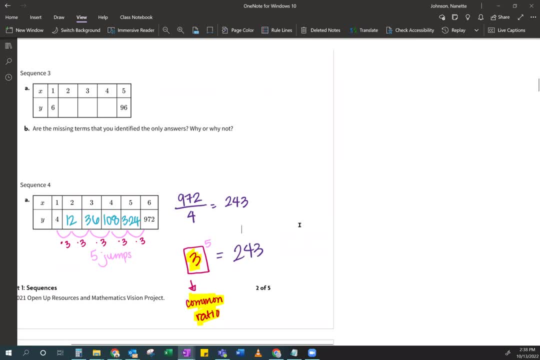 Um, so let's go over this so that we we get this in our brains, Okay, So the first thing we want to do is we want to divide. Okay, Dividing is not hard. It's something that you've been doing since. 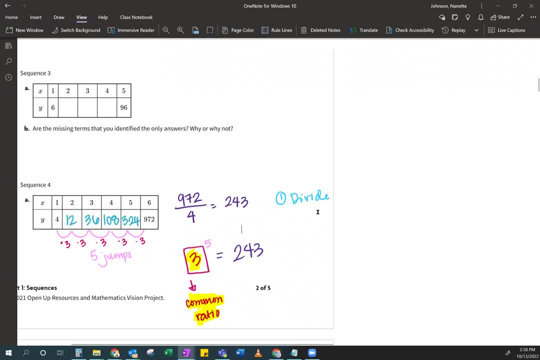 like fourth and fifth grade, maybe even third and fourth and fifth grade, right. So dividing is okay. You all are comfortable with that. The next part: this is where the level of what we're learning goes up a notch, right. So the next thing is- and it's kind of funny how I'm going to say this- is: 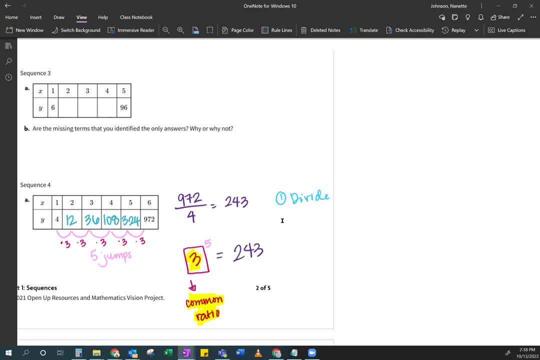 to kind of figure out. I want to write that equation that looks like something to the. something equals something. Now, there's a lot of somethings in my little equation that you can't see it, but the point here is it's something which is called our common ratio Shoot Where 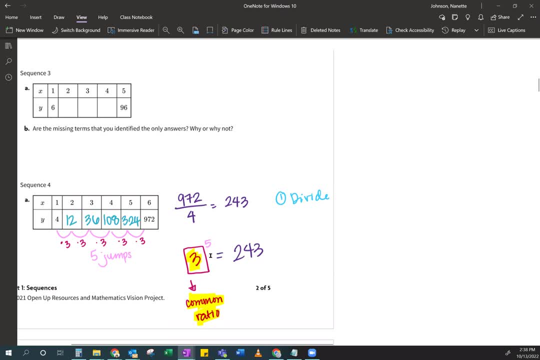 did I get this five again, You guys, where'd I get this five? Hmm, Oh, the five came from that five. Yeah, So this five here came from this five here, right? Oh, that doesn't look great.